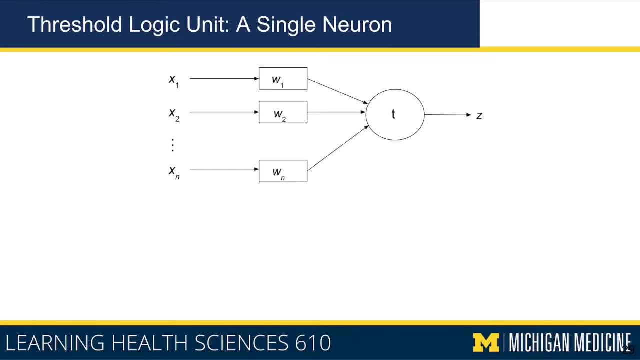 differently. and then you, you sum them up and see whether that combined signal is higher, is more than a threshold t. if it is more than a threshold t, then z is activated, so you, so the label would be one, otherwise it is deactivated, and so the label is zero. so an example would be: suppose you 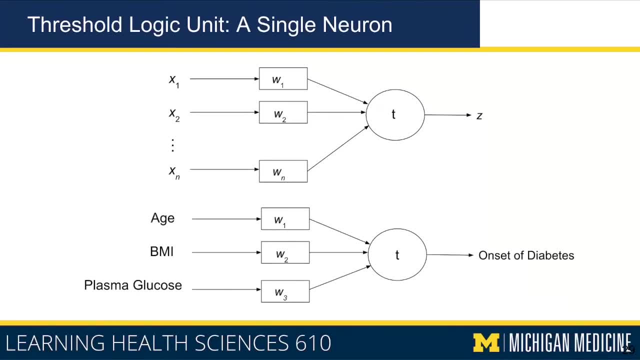 had three parameters: age, bmi and plasma glucose. these three features come in independently. you are weighting them differently. so age is weighted by w1, bmi with w2, plasma glucose with w3. and then, if this, if the total sum of this weighted- uh, weighted sum- is um above t. 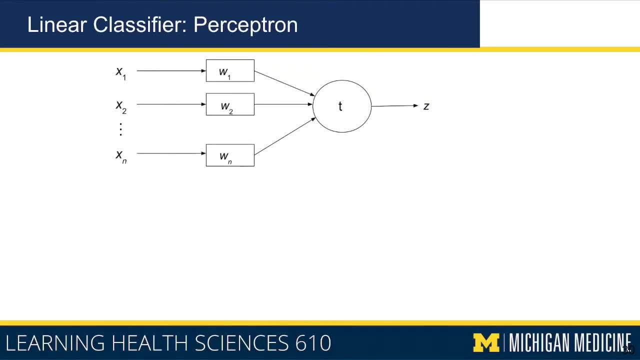 then you say that this person has an onset of diabetes, and onset of diabetes label is yes, um. so a classifier built on that idea is, uh, called perceptron. so again, you have x1 to xn as the features, which is weighted, and then if the weighted sum is greater than t, then the label is: 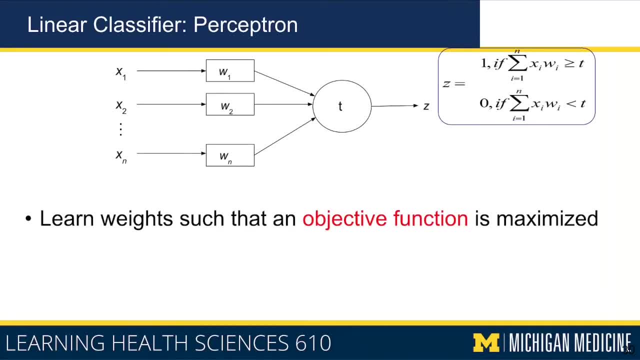 one. or if it is less than t, then the label is zero. okay, um, so that's great. so, so then you are now. now, the goal of this classifier and and training this classifier is just to find out these weights, uh, and you learn these weights such that the objective function is maximized in. 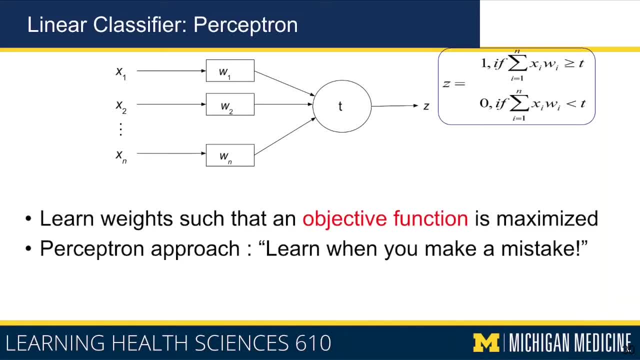 our case, objective function might be, let's say, accuracy of the model is is maximized, right, and so the the approach that you use to kind of train for perceptron is: you learn the model only when it makes mistakes. so if the model is maximized, then you can learn the model only when it makes mistakes. 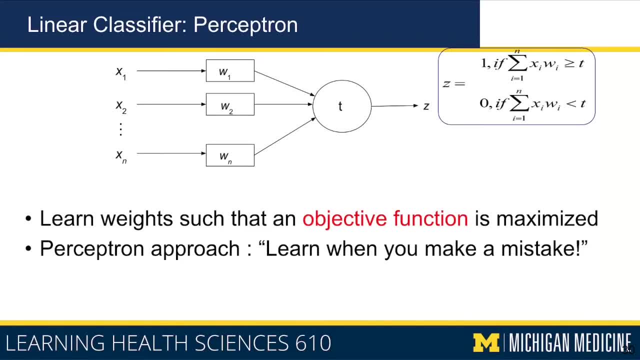 not making any mistakes. it is labeling exactly how your the training data is or how your label should be. great, you don't do anything, you don't touch it. uh, if it makes mistakes, then you will change the model slightly so that future instances similar to the one on which the model make a 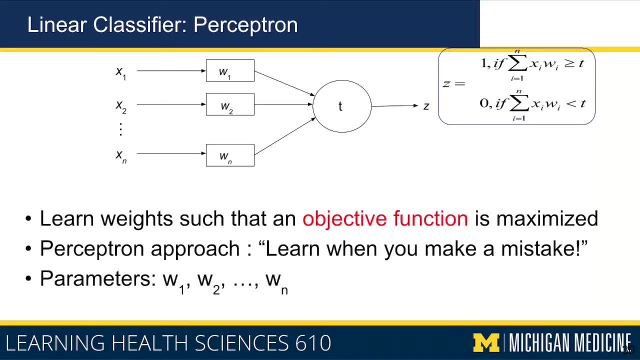 mistake will have less chance of uh, the model making a mistake on those examples. okay, uh, so so then the the goal is just to learn the parameters w1 to wn. but then, uh, what about t? is t a parameter if this sum is greater than 0.5 um and you make a decision and you have to change it to say if it's? 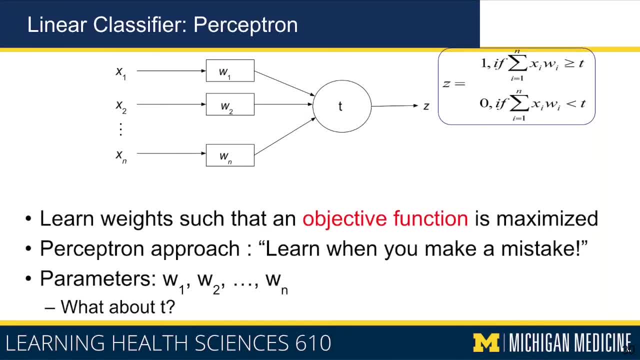 greater than 0.7, make a decision, then that value- 0.5, 0.7- is a parameter that you could also learn right. so, uh, what is common in perceptron and other models is that, instead of having that as a separate parameter, you can also learn that as a separate parameter. you can also learn that as a. 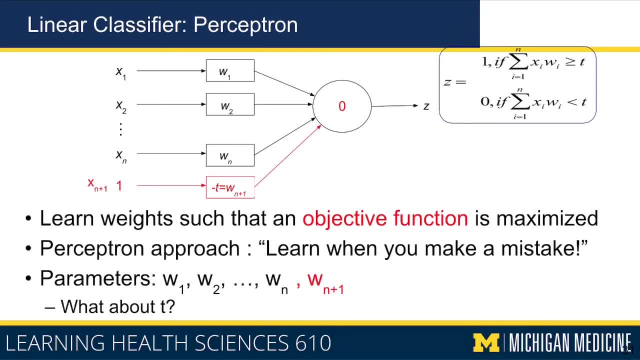 separate feature, you- uh, you merge it through into the other model. so what you then do is slightly change the option such that you use this minus t as an additional weight and the for an input. that is always one okay, and then the equation just kind of becomes: if the weighted sum of x1 to xn 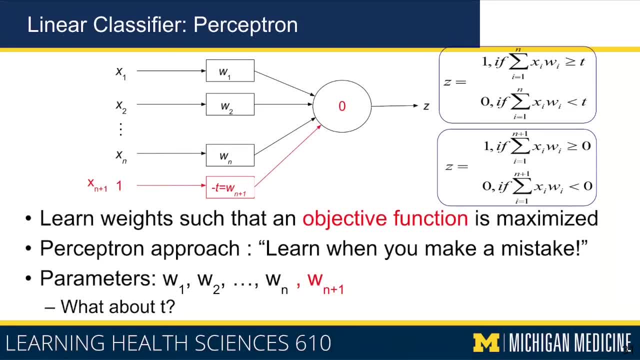 and one, this, this xn plus one, which is one, and then you can use this as an additional weight. and one is greater than zero, then the label is one. if it is less than zero, then the label is zero. so you have just kind of rearranged the uh, the math a little bit to just say that for any input x1 to xn. 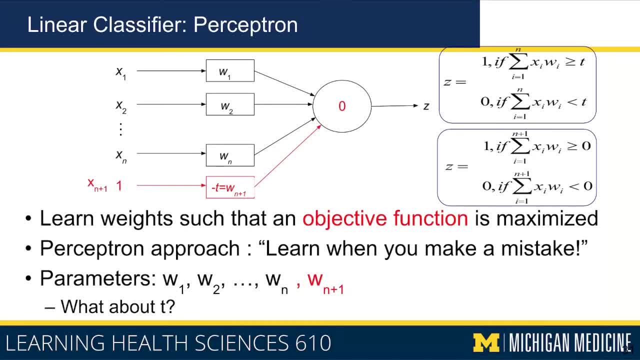 there is also this additional bias term. so even if the input is zero, if there is no input, there is this bias term, that can, that comes in and is weighted slightly and then you can you have some sort of a bias on where you can just say that x1 to xn is greater than zero, and then you can just say: 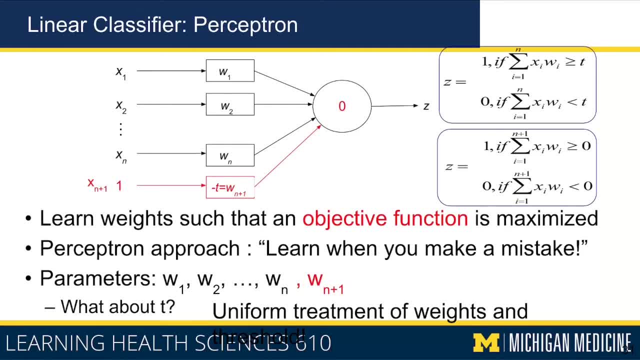 whether it will be labeled yes or no. okay, um, so this kind of gives us a uniform treatment of weights and threshold. great. so, uh, one thing that now you have seen here, and that is actually common in a lot of classifiers, is that, uh, the weight vector and the input vector are both now n plus. 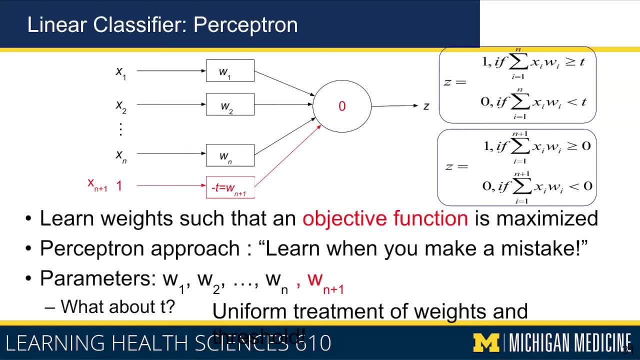 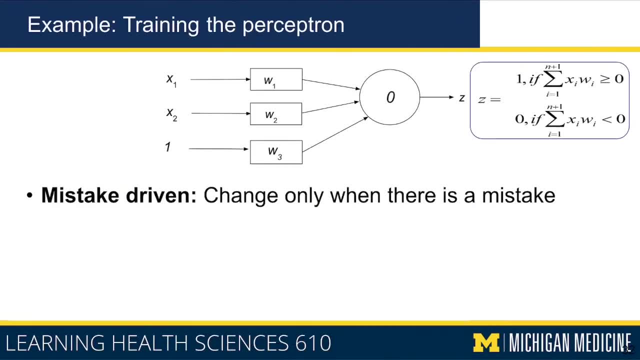 one dimensional vectors. okay, so they, they have a one additional dimension, uh, and that kind of represents this bias term. it's important because that is also very common in naive based models, where you have the input but you also have some sort of a bias term. okay, uh, so then, uh, the. the goal then is just to kind of train now n plus one, different weights. 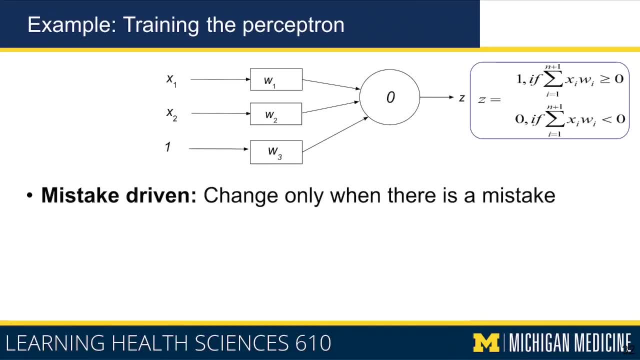 and you learn it only when the model is making a mistake, otherwise you let the model be okay. so in this example, let us kind of take an example where we have only two variables, x1 and x2. okay, just two numbers, uh. and then you have this bias term, so you're learning three parameters. okay, um, so because 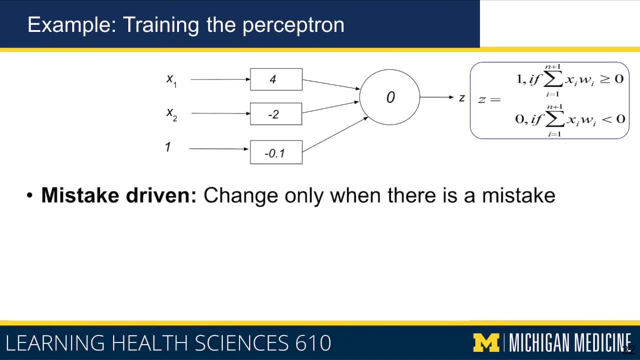 uh, the model is such that it it is makes a change only when it makes a mistake. you have to kind of assume a model, let's say the model where weight one, the one that that uh weights, the x1 is four, is minus two and the weight for the bias term is minus 0.1. okay, so for now the model is four times. 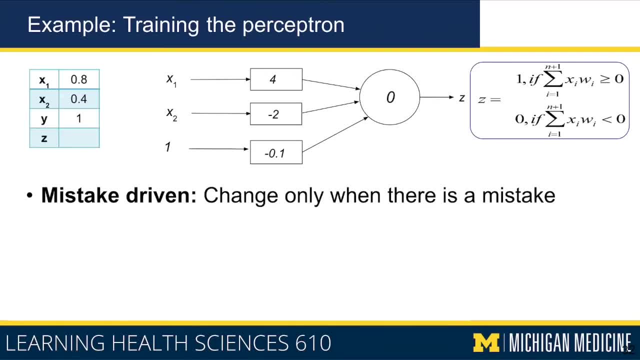 x1 minus two times x2 minus 0.1. if it is greater than zero, then it's a yes. if it is less than zero, it's a no. okay, great, so so, uh, you have the first training instance. the training instance is x1.8. 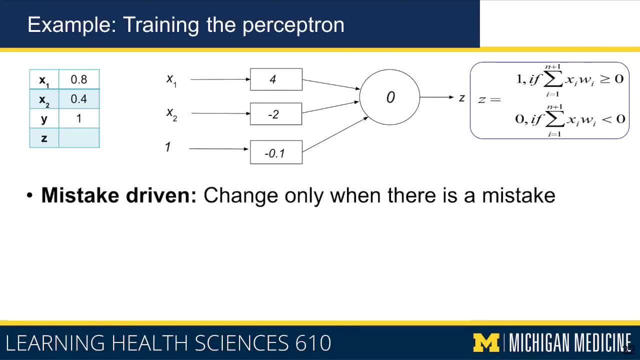 x2.4 and the label for the training data is uh one. if that is the case, then uh, what is the label? so you're going to say, for this one it is 0.8 times four plus 0.4 times minus two plus one times minus 0.1, and if you kind of uh do it, it's 3.2. 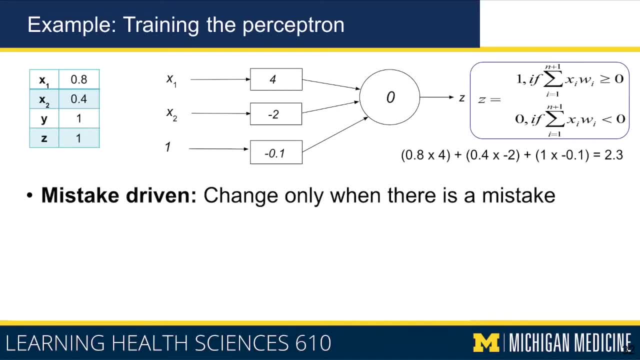 minus 0.8, that's 2.4. minus 0.1, that's 2.3. so 2.3 is greater than zero. so the label will be one, the. uh, the predicted label is one. so z is predicted label one. your actual label, uh, true label is one. no mistake, nothing to do, keep going, okay. uh, the next. 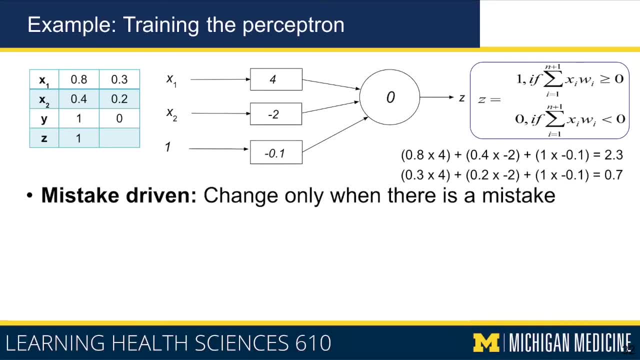 instance, let's say, is 0.3 x1 and 0.2 x2. uh, in that case, then again you'll do the same thing. so 0.3 times four, that's 1.2. 0.2 times minus two, that's minus 0.4, and then again minus 0.1, so 1.2 minus. 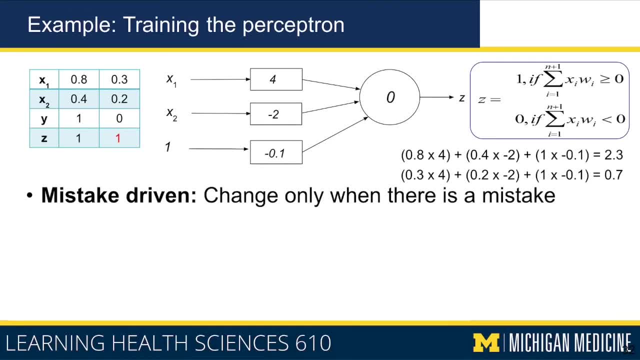 0.4 is 0.8 minus 0.1 is 0.7, so 0.7 is greater than zero. so your predicted label is one, but the actual label, the true label, was zero. so now they have made a mistake. so now that there is a mistake, the model has to be changed according. 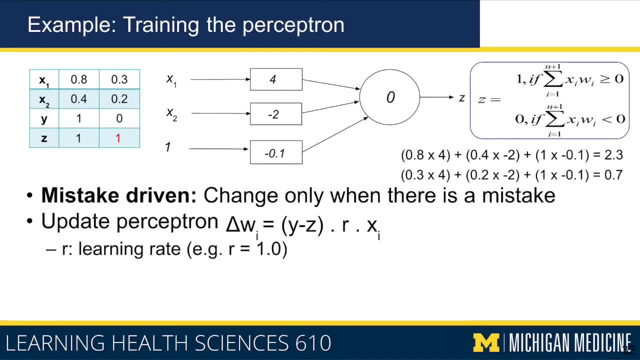 to the perceptron algorithm. so, uh, the perceptron algorithm is that you change it. so that means you change the weight. wy, uh, if you make a mistake. so y minus z, y minus z is, if a mistake has happened, is the actual label, z is the predicted label. if they are the same, nothing happens, it's otherwise. 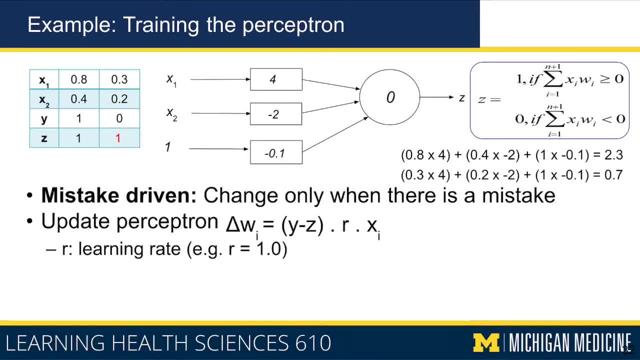 you're going to do it and then you have, uh, you if, if you know that you have to make a change, you make a change. uh, that is proportional to the input xi, and how much of input should you add or subtract? that is given by the rate of learning. so r uh, let's say, in this case, let r be one, okay. 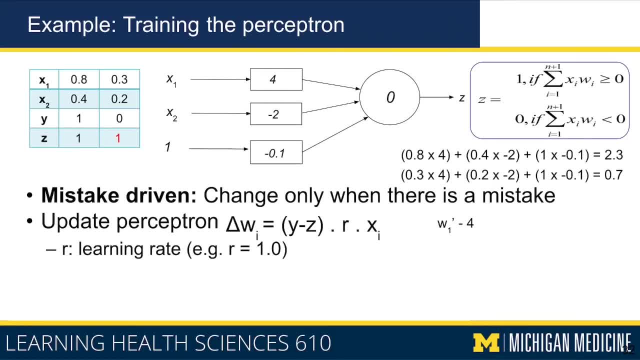 and then so what? what that means is weight one would be changed by, uh, by doing so, weight one, uh, the new weight one minus the old weight one, which was four, is uh, zero minus one times one. that's the rate times 0.3. that is the input. 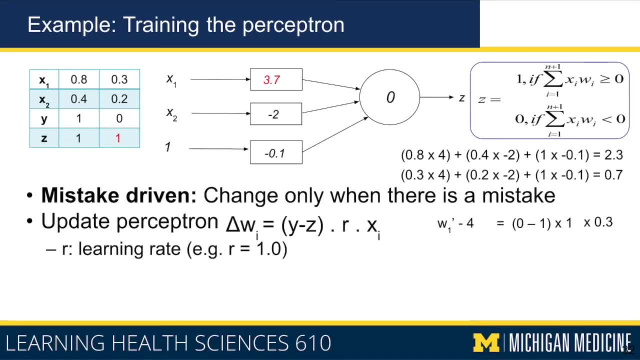 of x1, that, uh, that on which you made a mistake. okay, so then the weight new weight one would be, uh, four minus 0.3, that's 3.7. similarly, weight two would be given by weight two: the new weight two minus minus two, which is the old weight. 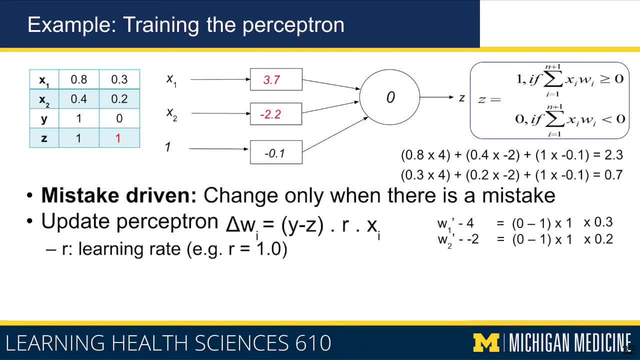 uh is uh minus one times 0.2. so uh, weight two would change to minus 2.2. what that means is it is: it is a minus two. you are going to remove or going to reduce it even more because it is. it was making a mistake, um, and calling something one when it should have been zero, so you have to pull it. 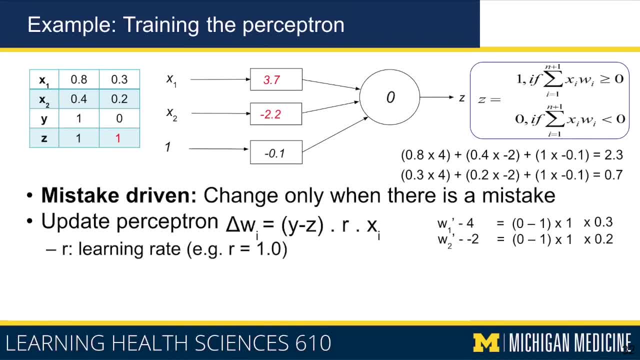 down. pull the weight down. so you're going to reduce it even more, because it is. it was making a mistake. make a negative weight even more negative. make a positive weight a little bit less positive. right, and same way here for the bias term: instead of 0.1, uh, it's now going to become uh minus 0.1 minus 1. 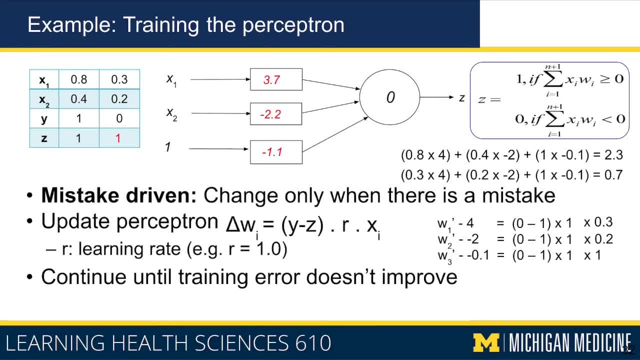 so that's minus 1.1. so now that we have done, uh, all the updates for all the parameters, you keep learning. you continue learning until the model doesn't improve or you're out of training data and that is your model: simple, uh, easy to compute, and that becomes your model. the advantage is perceptron kind of guarantees. 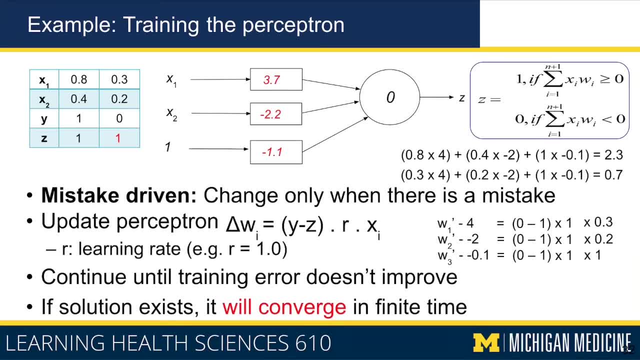 that if there is a solution, then perceptron, given enough data, would converge to a solution, which is a very strong statement. this is probably the only classifier that you have seen that is kind of giving you a guarantee that if there is a model that uh divides data. 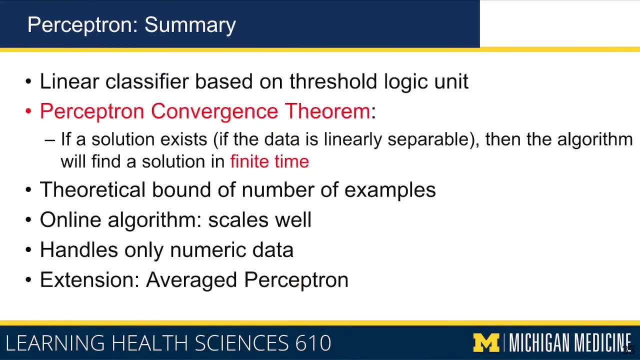 or or kind of linearly separates the model, that that is a valid classifier. this model will give you a classifier that will do the job, okay, um so, which is a very strong kind of assumption. so, to summarize, perceptron is a linear classifier based on a threshold logic unit. 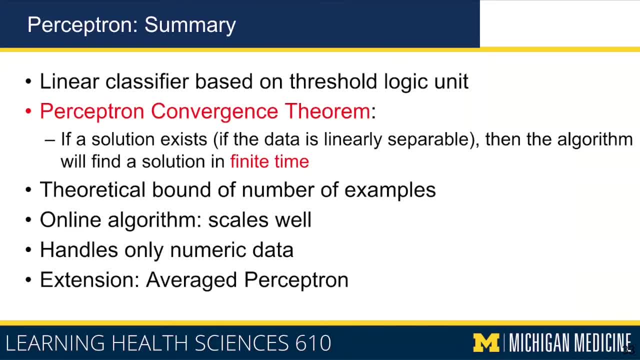 and has this very strong convergence theorem that if there is a solution- that means if data is linearly separable- then the algorithm will find you a solution in a finite time. note: that is a solution rather than the solution, because if there is one solution, there may be many other. 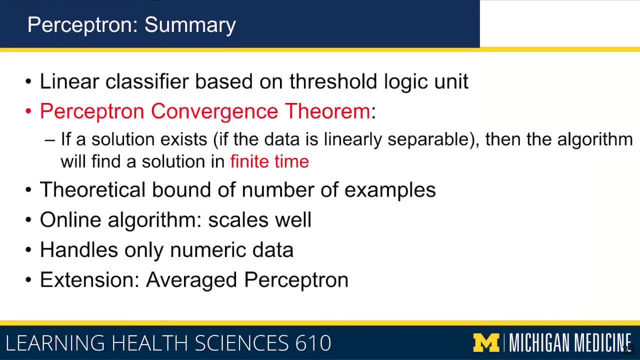 solutions. so so perceptron's algorithm says that it will give you a solution. it may not be the best solution, but it will be a solution for your model. uh, so it basically means that it kind of gives you a theoretical bound on number of examples, of how many examples you should see to get the model. 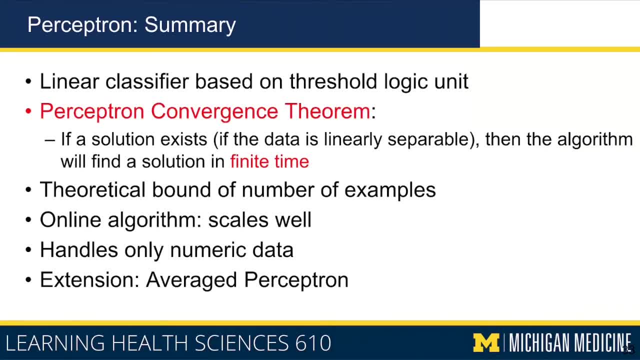 um, and because it's an online algorithm, which means that it only learns a number of examples, uh, as it sees examples, and if it sees a mistake, it makes a mistake on an example. so it's a very scalable algorithm and it's a kind of a. it can be trained in a batch way, and so on. uh, and the 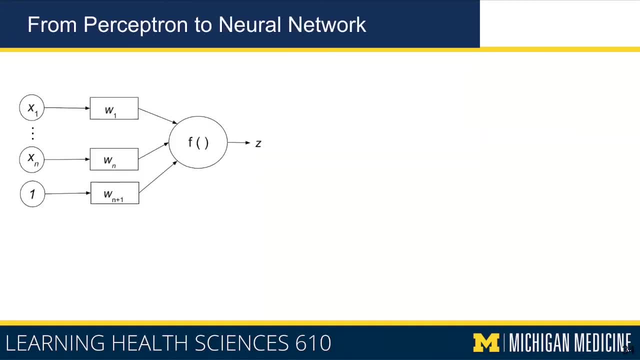 downside only is that it handles only numeric data, because it kind of creates a weight vector, so every feature has to be a numeric feature. um, how does this link to neural networks? uh, you start from the perceptron, but and it's the same kind of addition, just the way you have. uh, it's common to kind of give input, uh in circles, so x1 to xn and then 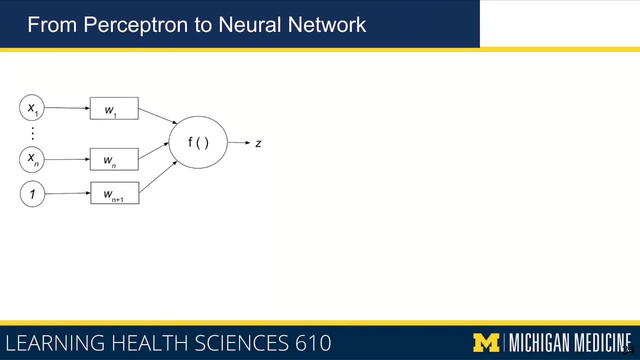 output, uh is also, uh is is the indicator and activation that goes into the next layer of input. okay, so x1 to xn and this bias term, uh, just the way you have seen it in a perceptron model. the only thing is here in perceptron we said, uh, that it was just a threshold function. so if it, 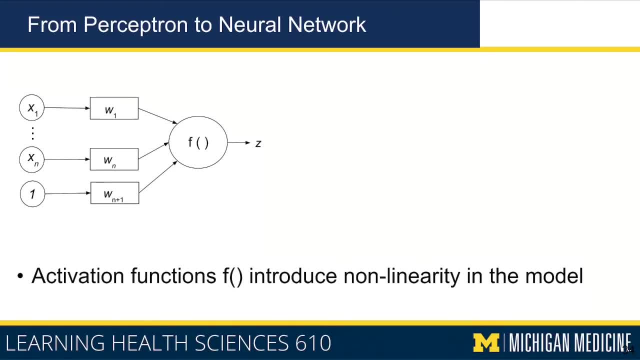 is greater than zero, the label is one. if it's less than zero, then it's a threshold function, the label is zero, uh. instead you can use an activation function, f, which is uh uh, different than just this sign. if it is greater than zero, it is plus, if it is less than zero, it is minus, kind. 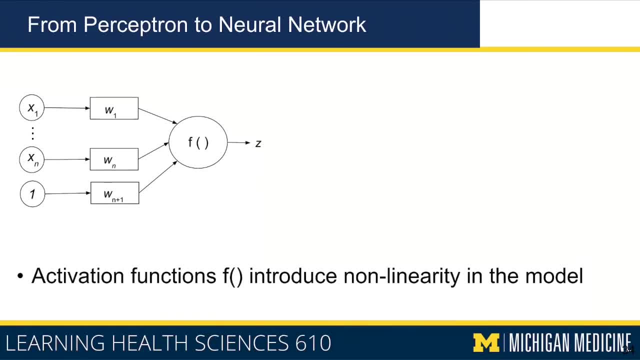 of a thing, uh, in sort of sign function. you can use some other function and this kind of introduces non-linearity in the model. so it does so that you can make this model as non-linear, uh classifier. uh, that is kind of important, especially because in a neural network sense it you the more. 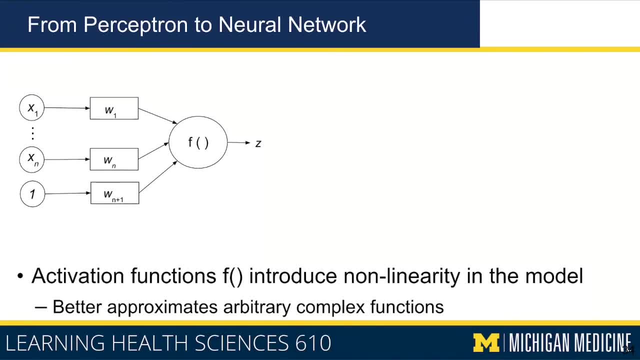 preferred kind of models, um are sigmoid or other uh, non-linear uh functions, and that is because they better approximate arbitrary uh, complex functions, uh. so the input then uh is the same as what you have seen. each one of them is a neuron and um. so each of these circles, the blue. 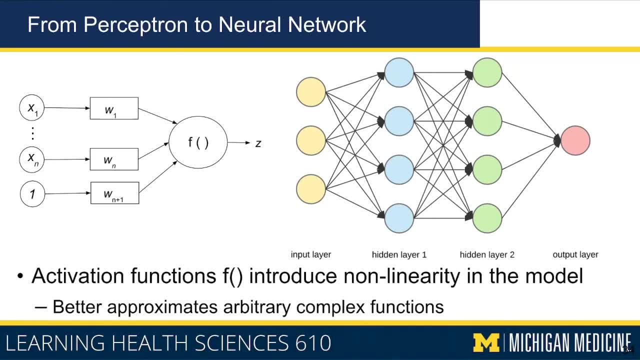 circles and the green circles are basically neurons and same as the red circle, um, where one layer feeds the next layer and the next layer feeds the third layer, and so on. okay, so when you have, uh, multiple hidden layers, these, these layers between the input layer and the output layer, are called hidden. 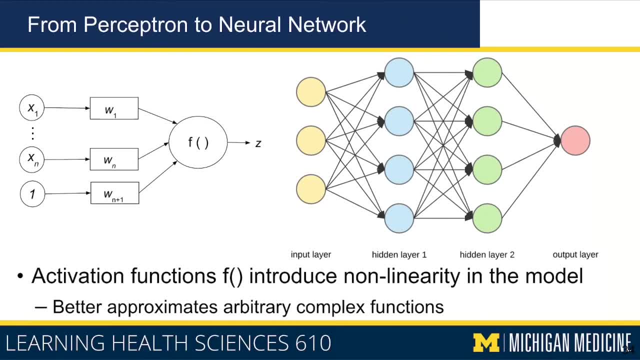 layers. uh, if there is more than one of these hidden layers, it's called a deep neural network model.